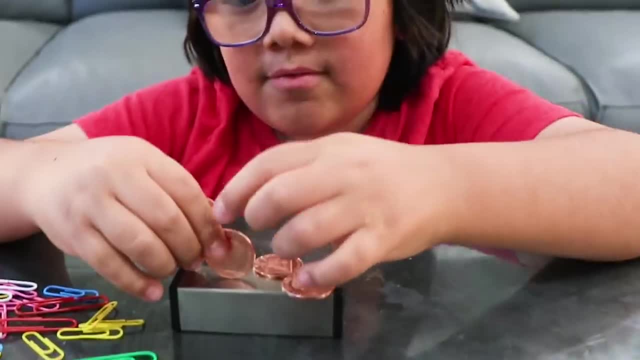 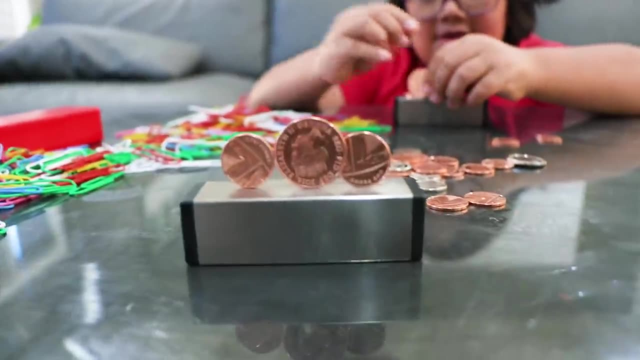 How high can you stack? This is hard, It is hard, huh. Okay, while you do that, I'm gonna try it too. How do they do this? Look, I got three so far. Ryan's still working on his penny. 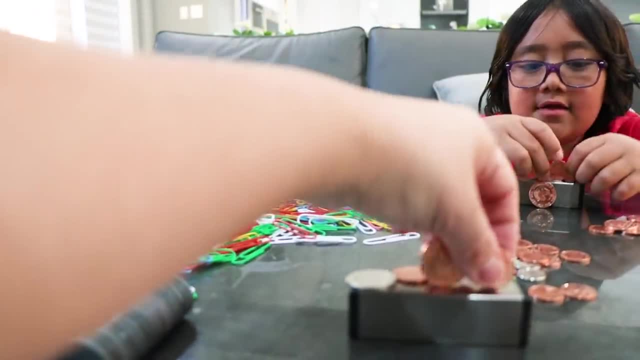 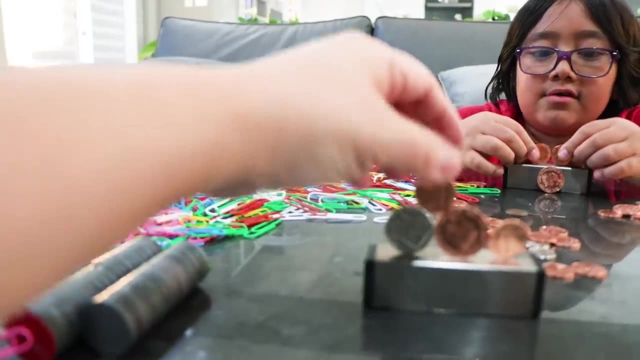 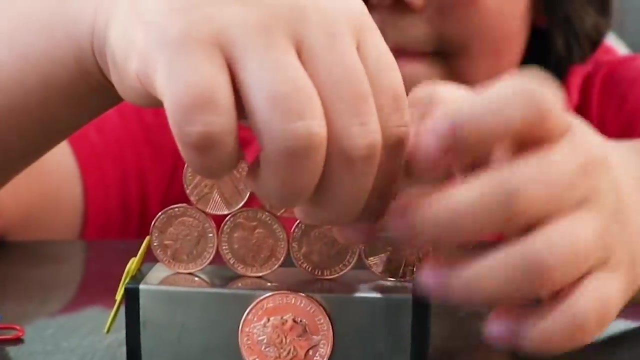 So hard. I know Whoa, mine keep falling. Yeah, Maybe we're doing it on the opposite side. Why would we Got it? Look at this beautiful Whoa. there you go, Looking good, Nice, Nice. 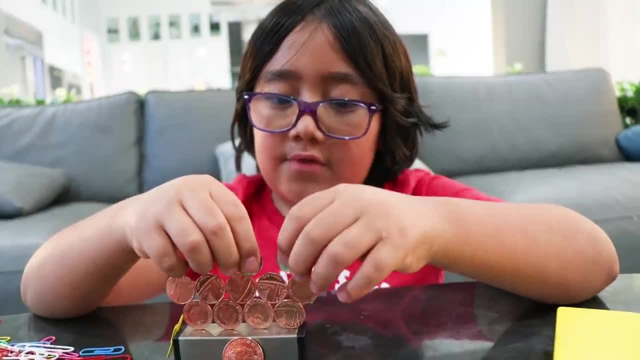 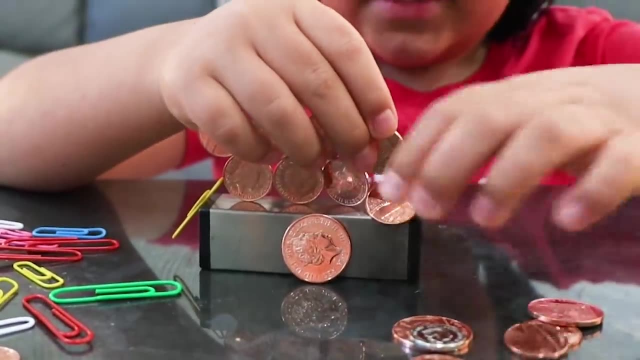 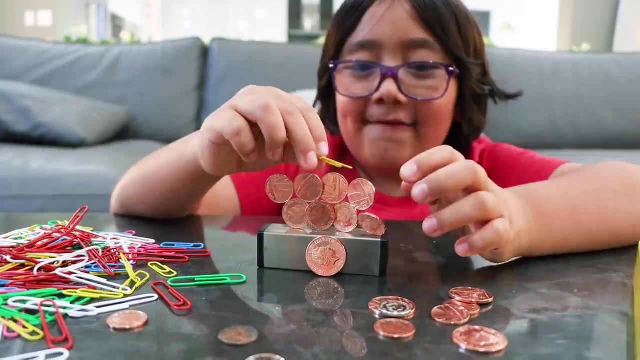 Nice. Oh, oh, these are too small. Ah, Mine fell Too small. Yeah, don't use those coins, Don't use these. Oi, oi, oi, oi, oi, Whoa. Oh, Okay, maybe this: 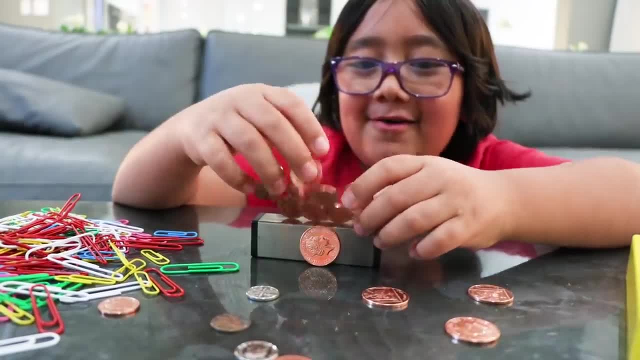 Ooh, There you go. Yes, Looking good. Oh, oh, oh, look at that. Yeah, Yeah, Next we're gonna stack it The blocks here. I want to show you guys this really cool trick, Okay. 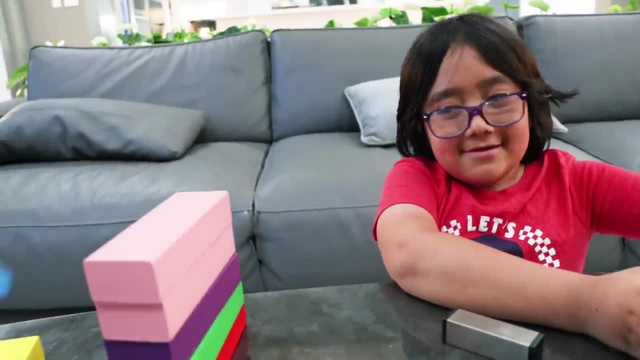 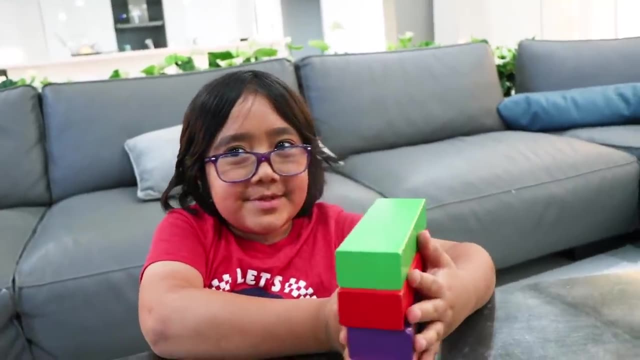 So I'll stack this side, Okay, Just literally stack it up, Okay. Okay, Like that, There you go. Wait, maybe I know what you're doing. I don't know 100%. Like that, There you go, Okay. 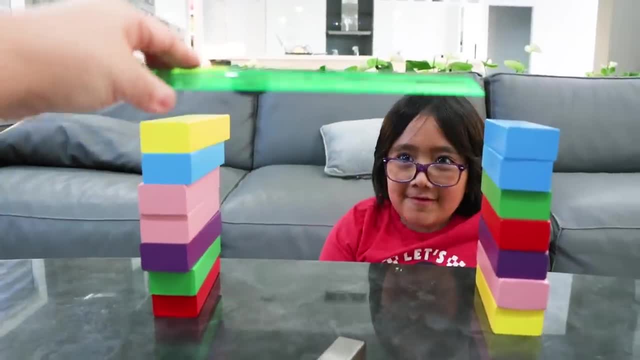 I have a ruler here where I put a magnet stuck into it. Okay, Now I'm gonna put this on top Here. hold this, It's gonna be like this. There you go, You can put it on top, Okay, Okay. 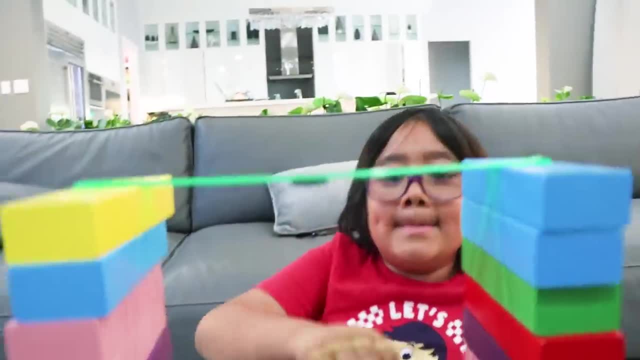 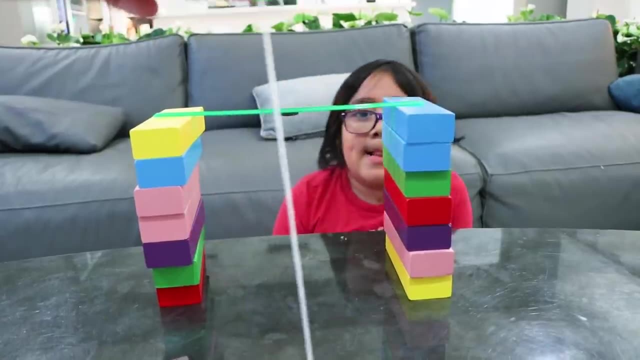 Okay, And obviously, Since the magnet is stuck right there, You know that a paper clip can just go to it right, Like so. You see the paper clip? Yeah, Then I have a string connected to a paper clip here. Do you see the paper clip? 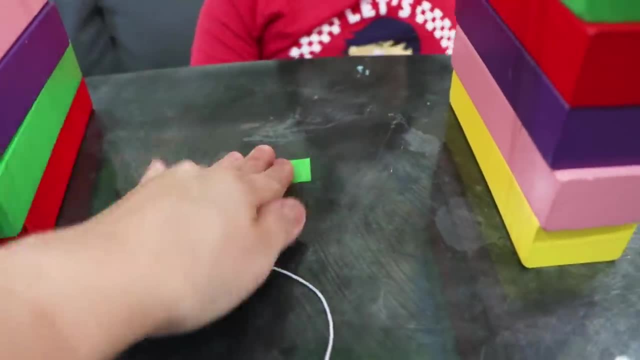 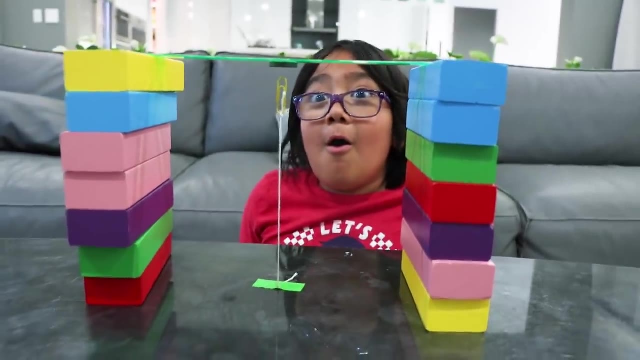 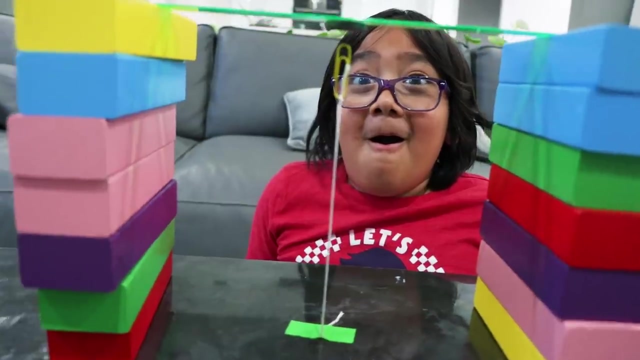 Okay, I'm gonna stick it to the bottom, Okay, Okay, Let it go. Okay, Let go of your hand. Did you see that? What happened? Look at that face. Do you guys see what happened here? What? Look what happened, you guys.